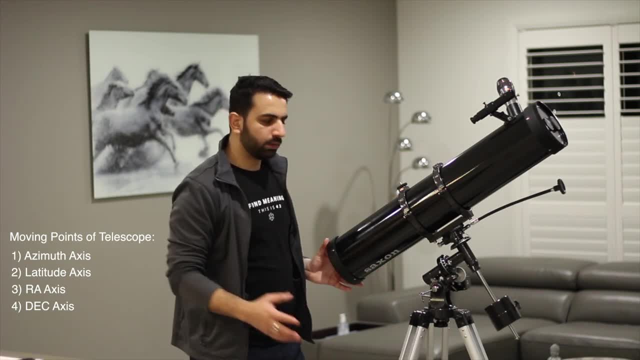 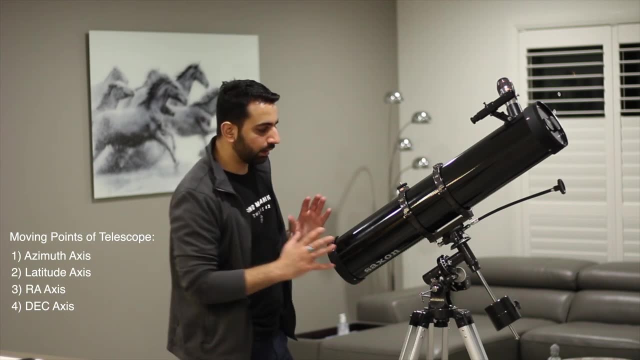 that it just, you know, just doesn't go everywhere. And if you further need to understand what is right- ascension and declination- i recommend you check out my other video, which i will link down in the description below. All right, so now that we understand what are the four moving parts of. 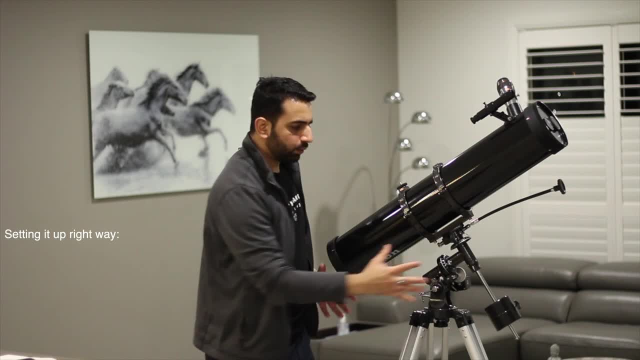 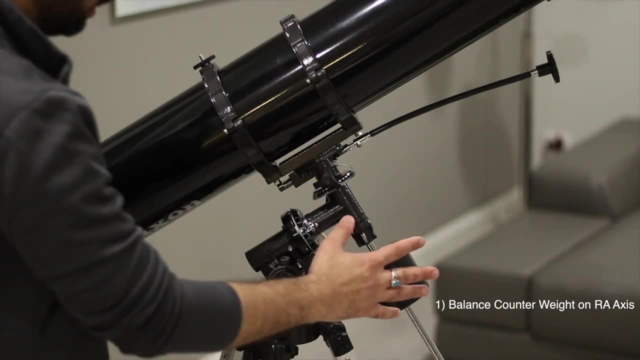 telescope. let's jump on to the point number two, which are how to balance the telescope and how to align the finder scope, which, in my opinion, is the most important part of understanding the telescope: balancing from the counterweight. so what we need to do is we need to loosen the wall here. 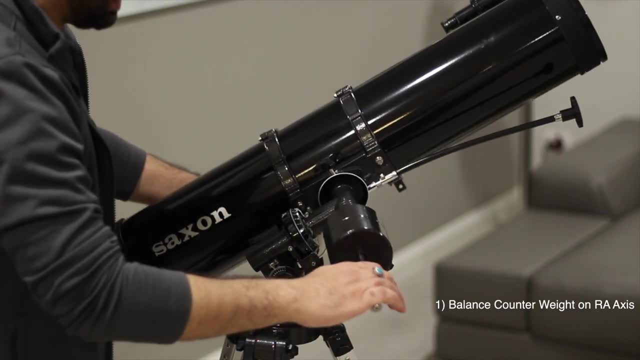 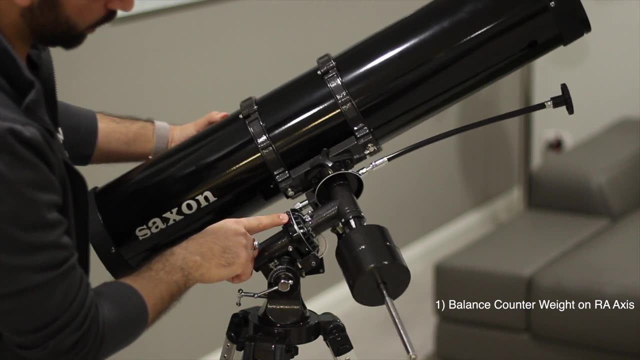 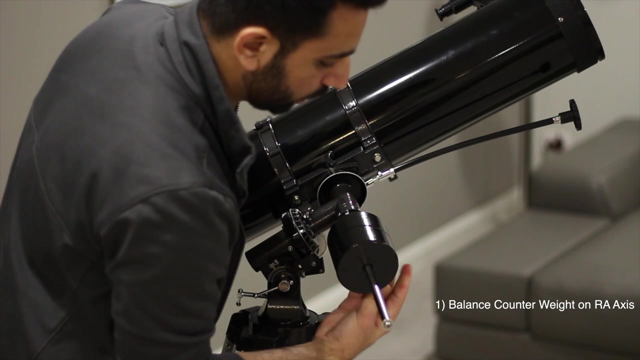 slightly, and wherever we leave the telescope, it should stay there to make sure that this is well balanced, and you can see we're just only moving the right ascension coordinate here. so at the moment it's it's terribly balanced. so what i'm going to do is i'll loosen it up from here and 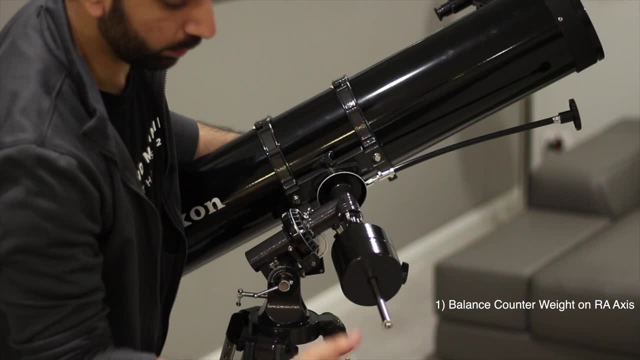 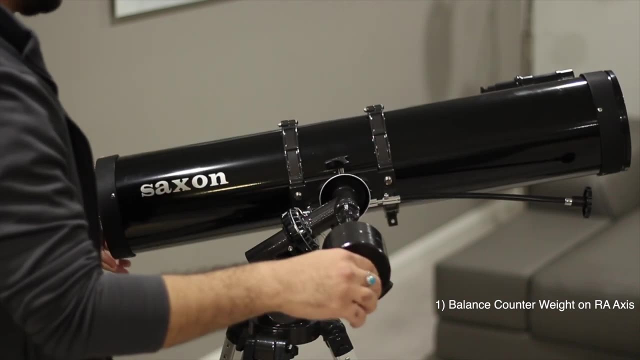 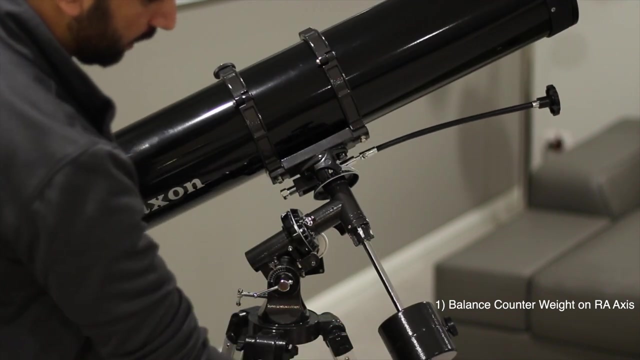 make sure the security screw is here so that you don't accidentally drop the weight on your foot. so i will kind of move it slightly so that it seems balanced. so, as you can see, after adjusting the counterweight, ra is just not moving. so wherever i just leave it, it just stays there. 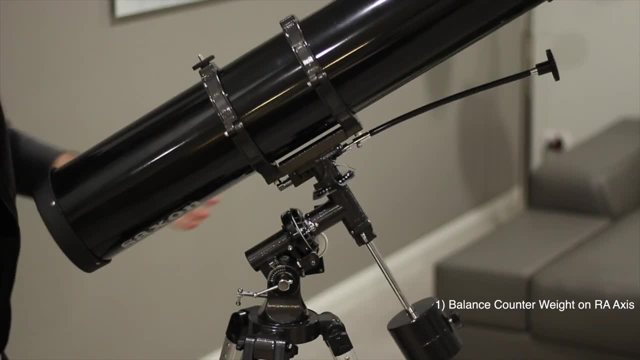 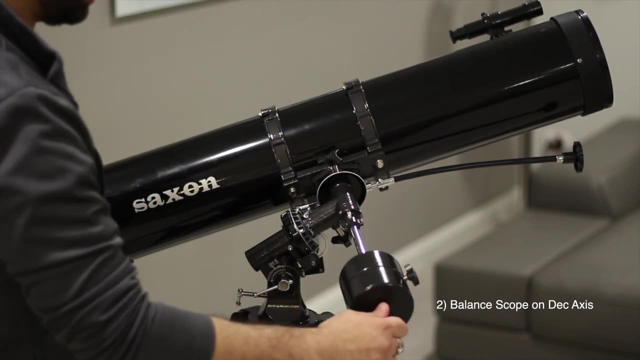 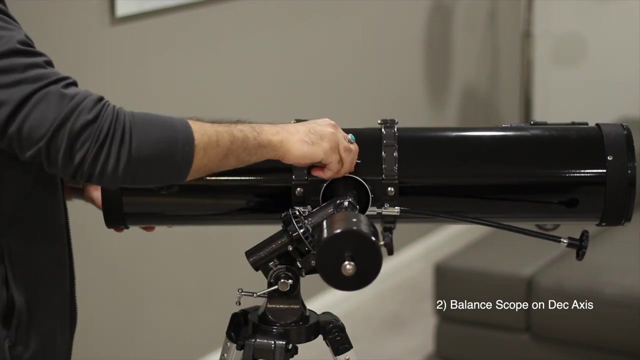 i check it on the other side to just to make sure the weights are all good, all right. so once that's done, we need to balance the scope, which is the declination coordinate. i usually like to put the ra on this angle like a flat angle, and i'm going to tighten the screw for ra and i will lose the. 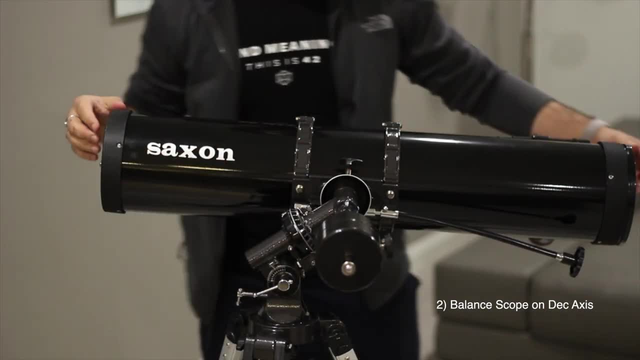 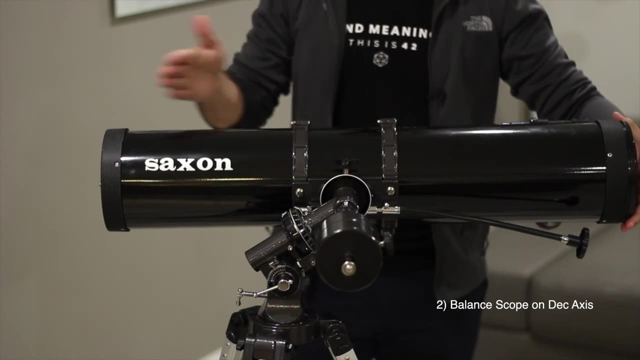 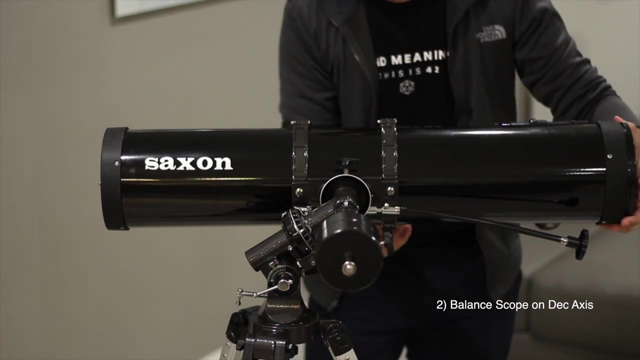 screw for declination here, so you need to make sure the scope kind of stays in the middle. as you can see, it's kind of leaning here so we need to move the telescope a little bit back. so i will loosen the uh screw on these clamps here and we'll just move it slightly back. 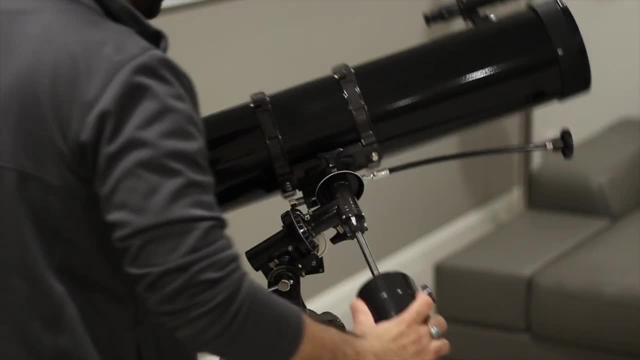 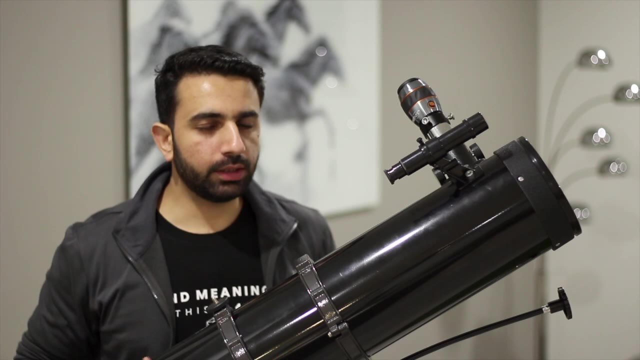 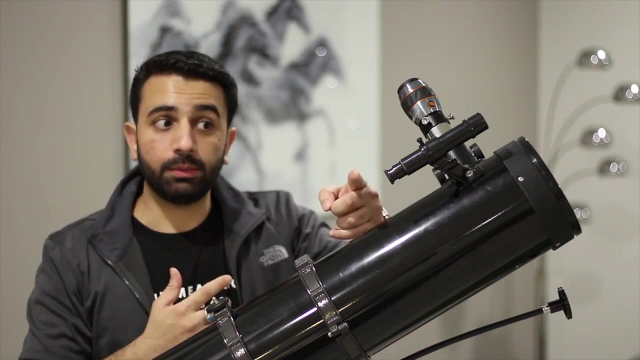 and we're done all right. now let's talk about the notorious final scope, and this, in my opinion, is arguably the most important aspect. i mean, you can get everything right in setting up the telescope and you've not aligned this perfectly or it's a little bit off.